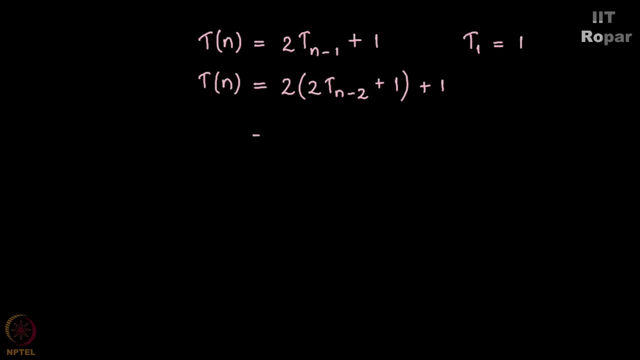 one as plus 1 as it is Now. I can further simplify this as 2 square Tn minus 2 plus 2.. I have just expanded the bracket and written multiply 2 throughout. Now Tn minus 2 can be further written as 2 square 2 times Tn minus 3 plus 1 and the rest of plus 2 plus. 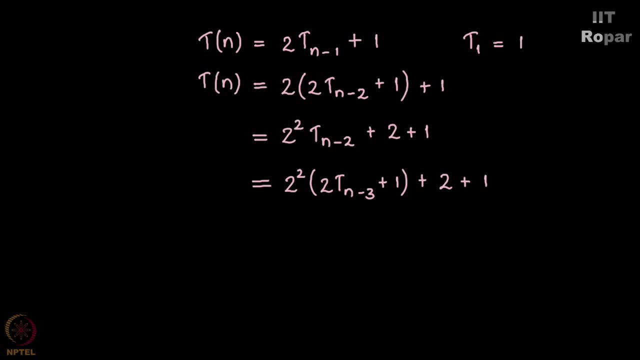 1 remains. as it is Simplifying this, We get T of n as 2 cube, Tn minus 3 plus 2 square plus 2 plus 1.. If you are probably not understanding, you have to stop or pause the video, pen down things yourself and it. 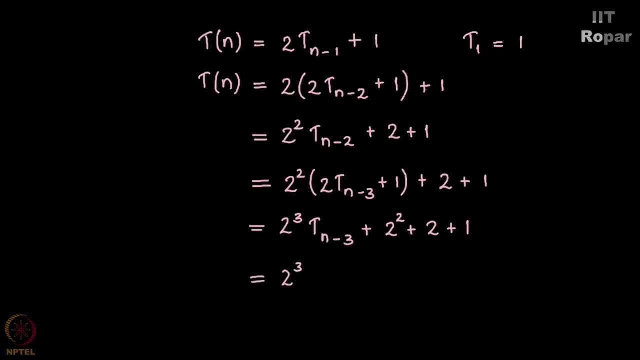 will be much clearer. The next is as usual: Tn minus 3 can be written as 2 times Tn minus 4 plus 1 plus 2 square plus 2 plus 1.. This becomes 2 to the 4 Tn minus 4 plus 2 cube plus 2 square plus 2 plus 1 and the process. 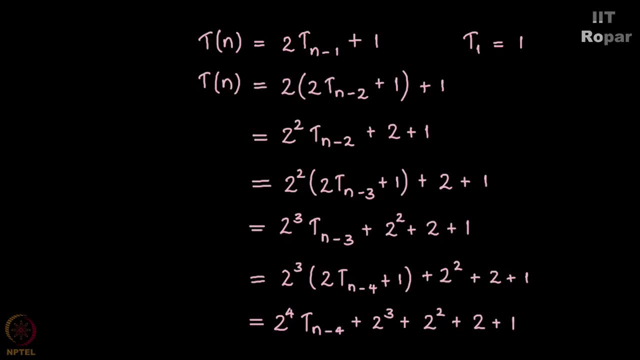 continues. So what can we write in general? In general, Tn can be written as: 2 to the rTn minus r plus 2 to the r minus 1 plus so on, plus 2 square plus 2 plus 1.. Now we know that T1 is 1.. 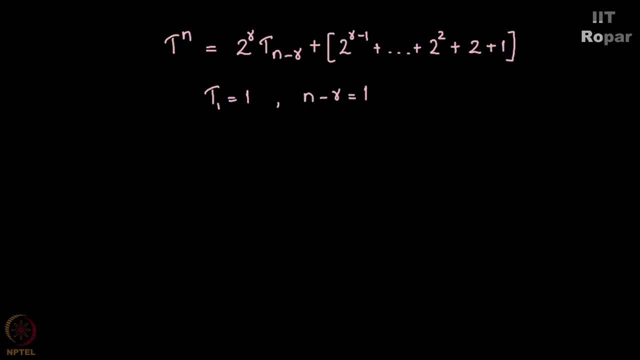 1,. this was the initial condition, and if I have to write here as T1,, I write n-r equals 1, and hence r is n-1,. I have just taken r to the other side, so r becomes n-1.. 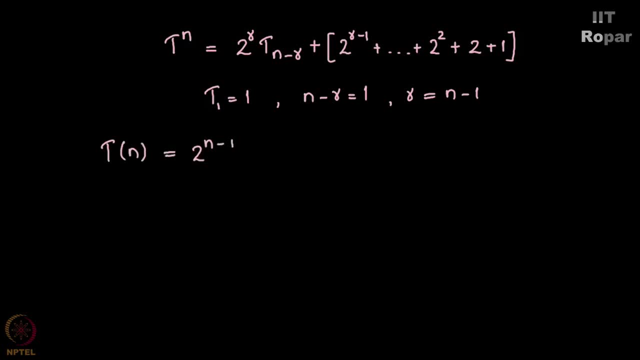 Now I can write T as 2 to the n-1, in place of r, I am going to substitute n-1,, so it becomes 2 to the n-1, and n-r becomes 1,, therefore it is 2 to the n-1 plus 2 to the n-2 plus. 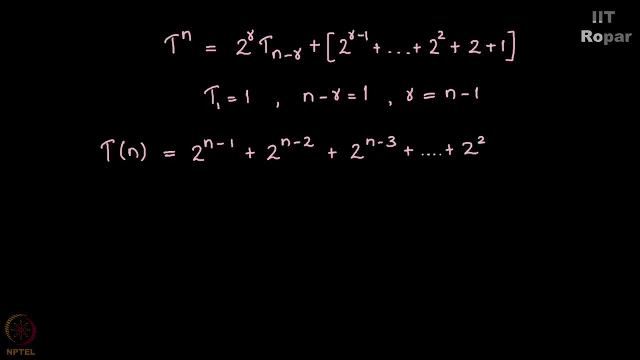 2 to the n-3 plus so on: plus 2 square, plus 2 plus 1, and for simplicity or for calculation, I am going to just substitute T as x. we are going to simplify this and I'll substitute back as T. so now for simplicity, let me write this as x.